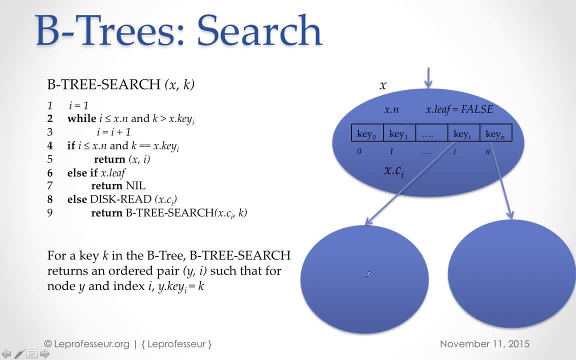 the key may belong to? which children or a sub tree? uh, if the key is not found at an internal node, So what? it is basically here up to line number one, two, three. that basically finds the smallest index i, such that there is a key k existing between that node and the tree. Now you need to 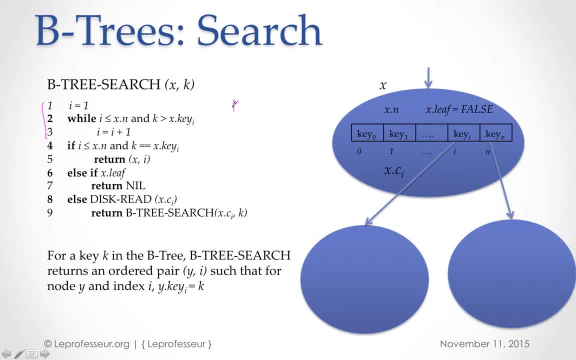 that says that your K, your key which you are trying to find belongs to, is less than X dot key key at a particular index, less than or equal to. so what it means that once you know that your key is less than particular index key, let's say K. 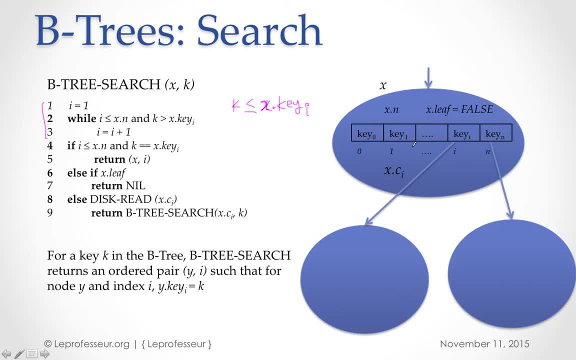 Yi, and if, if your K key is not found here, then what you can do, basically you can descend to one of the sub sub children. and so, basically, here is that if, if you find, then you return that particular node and the index D and which K is found. but, however, if it is not equal to, then, if this is a leaf node, then you say: 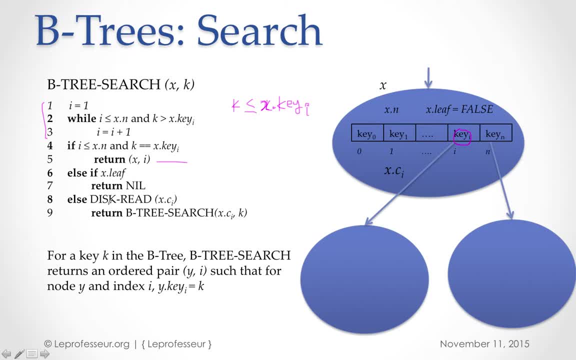 key is not found, and if it is not a leaf node, then what it is? you recursively find the key k in the sub children of that particular index: x, c, i, k, right, so basically what it is that. so key acts as a, as a separating, uh, as a separation of the sub crease. so you might have. 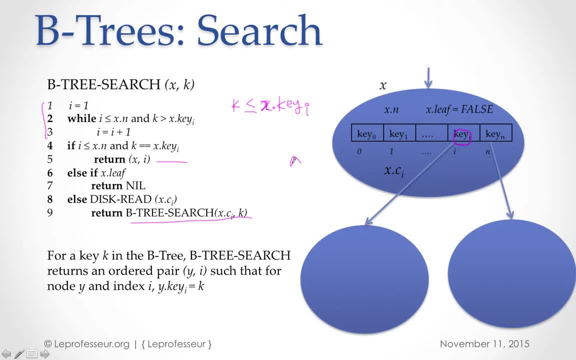 let's say, if, if the a, b, you have the children keys and so what it is here. if you have c and e, okay, so now here you may have b and you may have here f and g, and you are trying to find d or you are trying to find basically b. 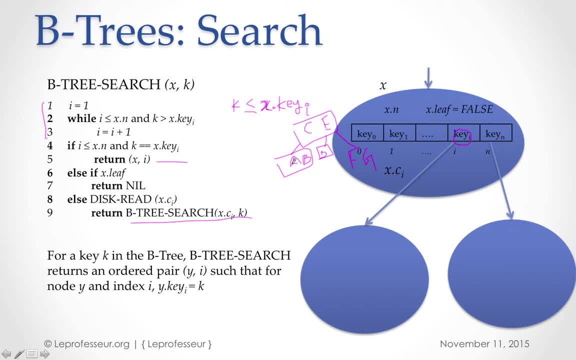 so what? it is that if you find that the b is less than equal to c, so you just descend to the first children and you'll find the key here. okay, it's a very simple algorithm. now notice that. what is the complexity of this algorithm would be, let's say, if your height is h, 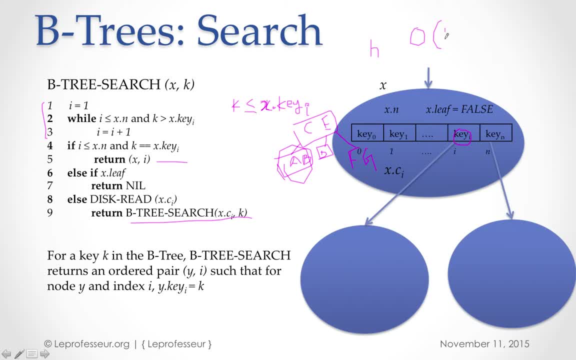 then this algorithm will take o in bigger notation, t, h time, or you may also write it as o t log base, t and n. that is the operation it will take where n is the number of keys or your index is at a particular internal node. okay, now let's talk about the creation of the tree. 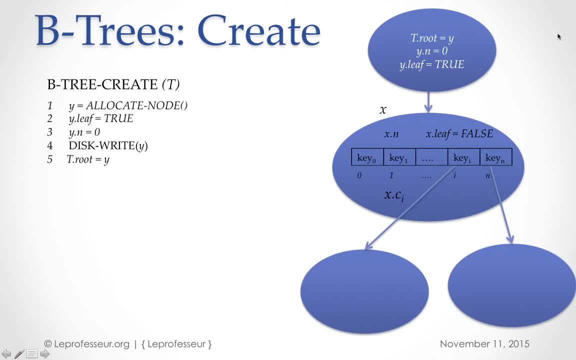 it's again a very simple procedure that once you know what you're going to store at each node, then you allocate the node or in in allocate node processor. basically it is allocating the memory space. that memory space can be a page or can be just simple, simple node or simple memory. uh, by its. 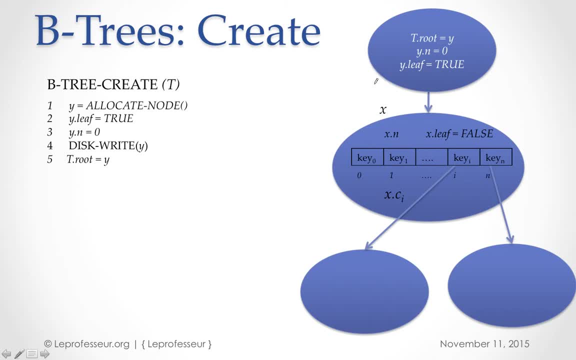 way like this: uh, a node typically will have, so node will have how many keys, whether it's a leaf node or not, true or false- uh, a array structure or link to its structure to store the values of the keys and the pointers. so these are pointers to the children's okay. 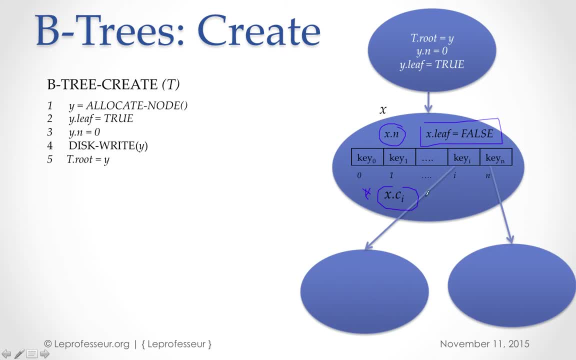 so remember this key acts as the separating is. so whatever are the children's, sub children's of this tree, so the left sub children say KEYI, means that all the values, all the keys in the sub children will be less than KEYI. okay, and on the right sub children will be more. 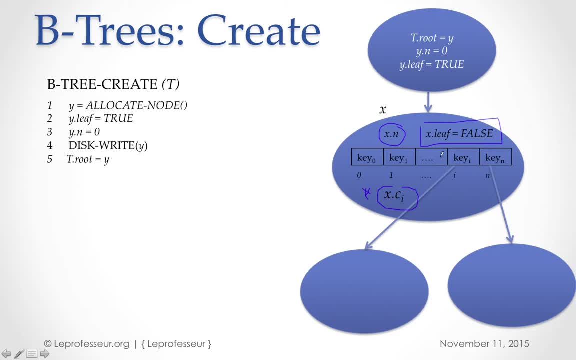 than KEYI. so that is the structure which is which is for B trees. so, no matter what we do, we do insertion, orAt least then we have to preserve this structure at every internal node. these keys are stored in an non decreasing or increasing order. okay, all right. so once you have you allocated that you. 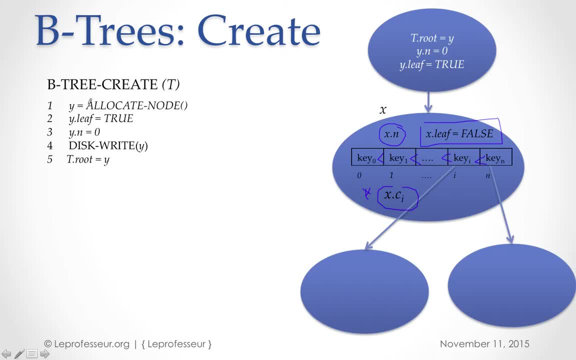 basically notice that LEAS font itself is not in the row and that's not track. create a node and once you allocate a node, you get the pointer to the to that particular node and since the tree is empty, you just select that particular one node as a root node. okay, simple process. now insertion is a bit. 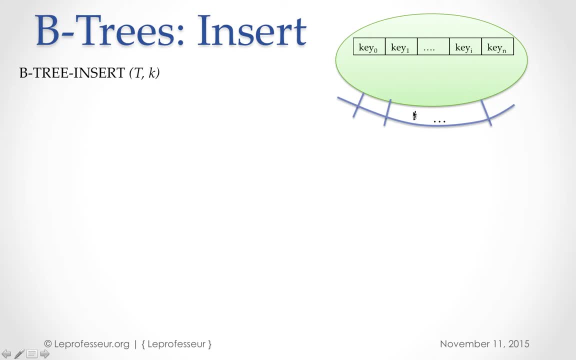 tricky operation. okay, remember we discussed about what is T, is the, the order of the of the P tree, and if the keys are restored at each internal node in an increasing order and that order is maintained. so basically what? whatever are the sub children's, so left sub children of this free left? most will 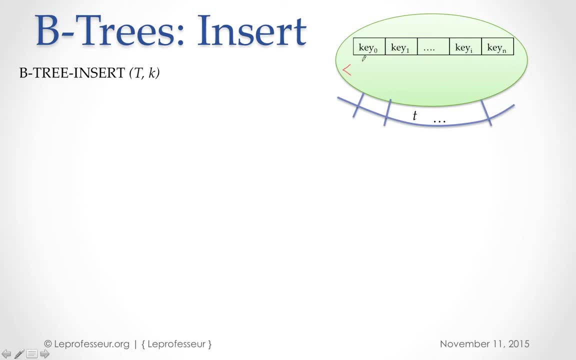 have all the keys less than key 0, and then the right children, next children left most, and then the next children will have keys in between k y 0, greater than k y 0 and less than k y 1. okay, and next children will have k y 0, greater than and less than k y 1. 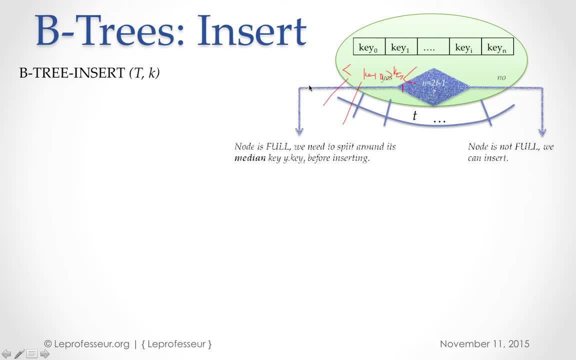 so that's, the structure is preserved. now we have the case, in interesting case, that if number of keys n is equal to 2t minus 1, what is the 2t? 2t minus 1 is the maximum keys this node can have, okay, and if we want to insert another key at this, 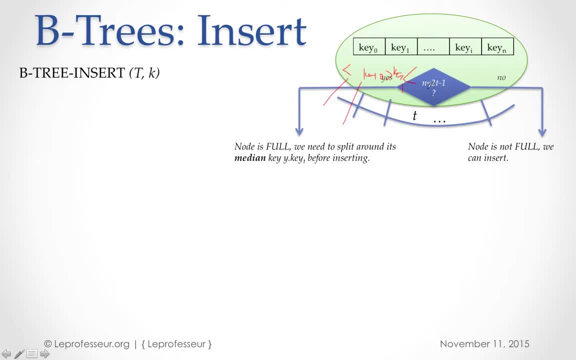 node. how do we do that? so we have to first check the number of keys stored at this internal node is equal to 2t minus 1. then we have to split that node, otherwise we just simply: node is not full, we can insert, okay. so let's, let's talk about how, how the splitting walks. 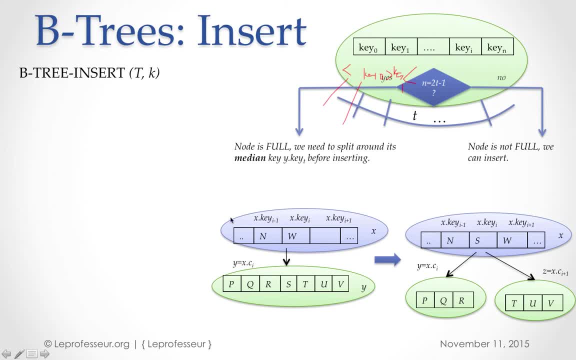 okay, before getting into the detailed algorithm. so let's say you have this Y node, okay, and you, you have this Y node and this node is full means it has 2t minus 1 keys. with the 2t, it's its children. okay, what we're going to do, we're going to 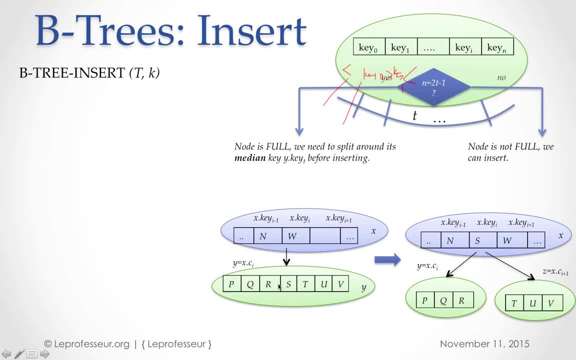 we're going to get its root node. okay, this, this nodes root node. okay, I say this is structures. root node is this one, okay, so how we're going to split it. so what we're going to do, we're going to find a median key, okay, which is s here. 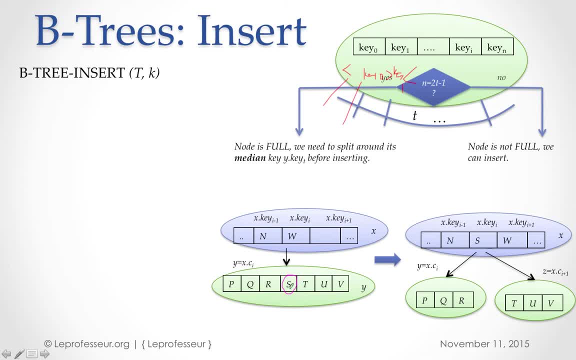 the middle middle key and move this middle on to the root. it's sub trees root. read root keychain. okay at appropriate location. okay. so let's say we have n and W, so s will fit between n and W. so we move s on to the root and s will fit between n and W, so we can move s to the root and s will fit. 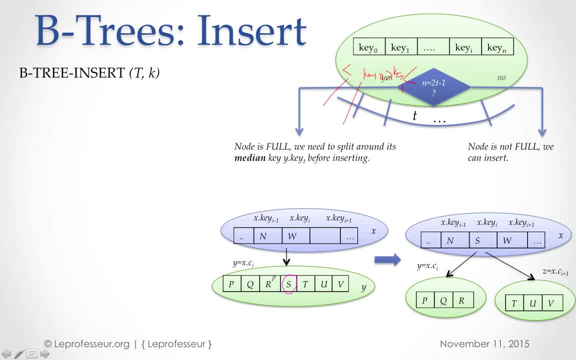 between n and W. so this is the n and W. so this is the node. and this node is split into two nodes. so one will have PQR keys and another will have TuV. so these, the new node, is split into two. now these two becomes the children of its 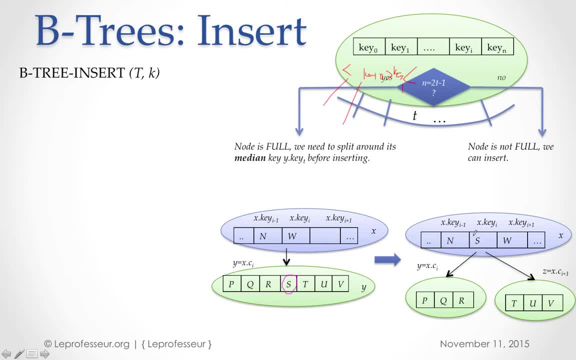 parent node and how its gonna store that the keys, the parent node and the parent, the keys which are less than s, will have pointer xci, y, equal to xci and a new node, whatever number of whatever you know keys which are greater than your s will go into the new children and that new children. 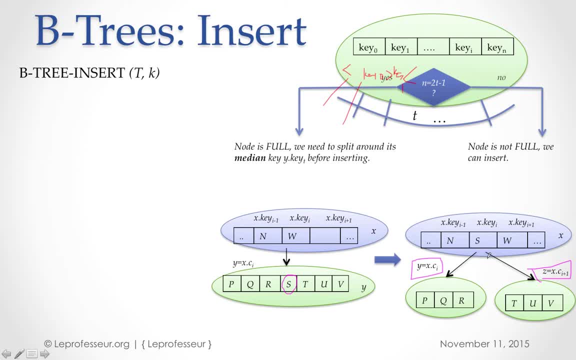 will be added, so its pointer will be added to the parent node. okay, so let's talk about the precision. okay, so it's a very simple processor that initially you say that whatever is the t to t dot root and you assign it to r, you know, and one here, line number two: 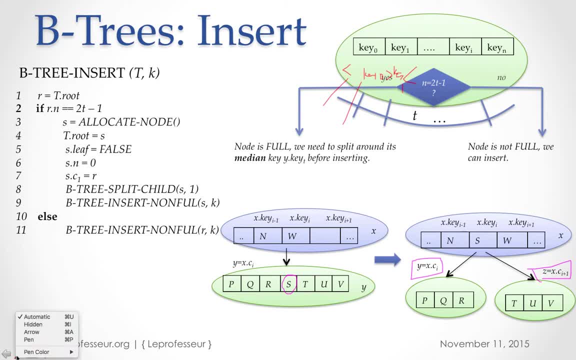 to nine. basically, you are deciding here whether this, uh, this node in which you are gonna insert this key- okay- is full. if it is full, then you have to create a new node. okay, you have to create an extra, you have to split it. so it means that you are creating a new node which will essentially become: 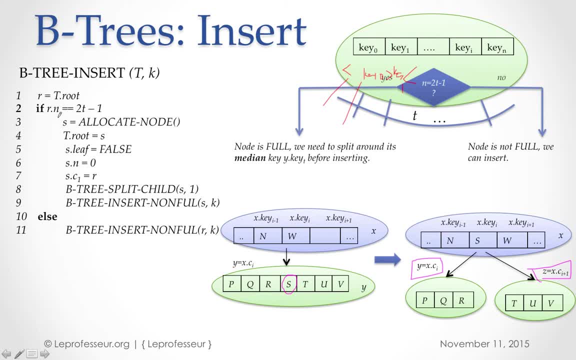 another children, okay, so that that basically is doing that job. and then this, this processor is splitting, splitting the child. child is nothing but the, the child of its parent is this one. so this node is getting splitted and then, um, you can insert this key, okay, into the non-full node. 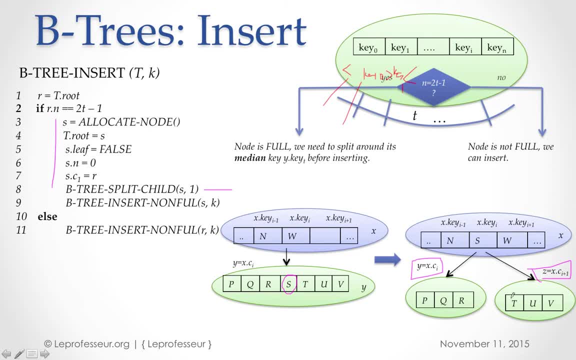 so this becomes non-full node, okay, you know. so now you want to insert over here. okay, otherwise, if your node is not, it's not full, then you just execute non-full procedure. okay, interesting enough. so now these two into two processors is split child and no full. 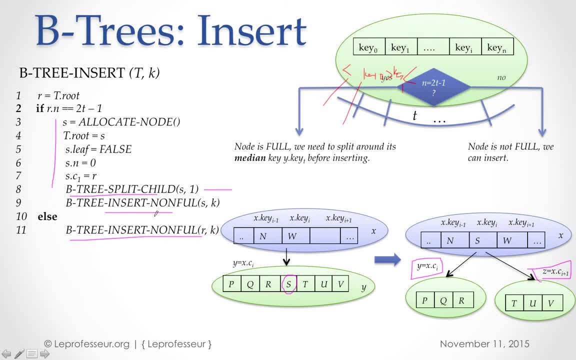 these are the key things which will determine the complexity of the process. so now let's talk about this algorithm. okay, so remember, these procedure are recursive procedures. we discussed recursion in in past lectures. it's a very beautiful technique. recursive, you know, doing the computation recursively. write once and use that algorithm recursively, based on different input sizes. 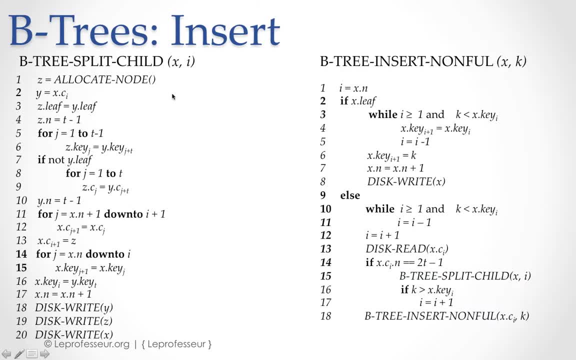 all right, okay. so now let's talk about the split child procedure first. so what it is that split child processor, what it is that it will take, say node x and an index, i such that, so that x- okay, this nodes children x, dot c, i for a corresponding index is full okay. 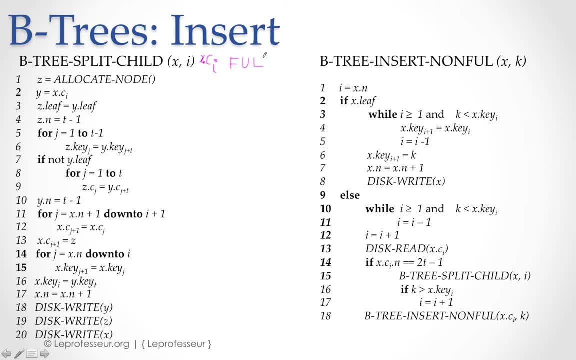 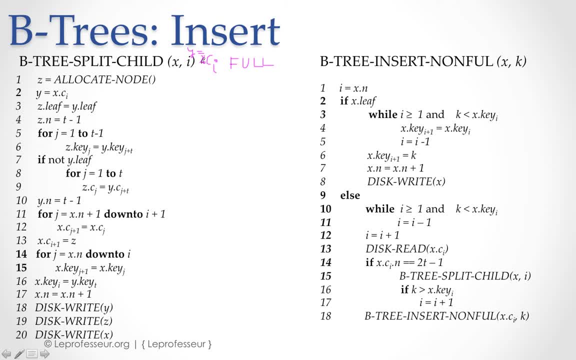 But now, after splitting, it will reduce to the t children and t minus 1 keys. So 2t children, 2t minus 1 keys. Now it will reduce it to t children and t minus 1 keys. 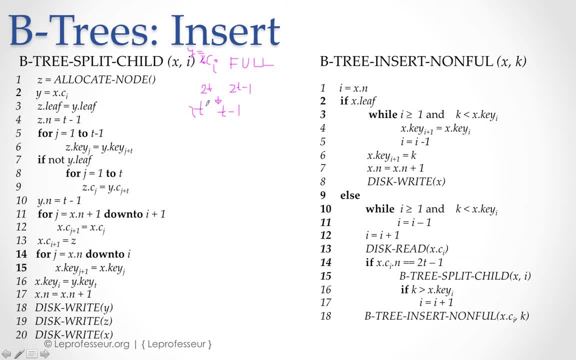 After splitting, after splitting so that one will become y and z will become similar y, You are splitting into 2 and t minus 1 keys. So line number 1 to 9, this is line number 1 to 9.. 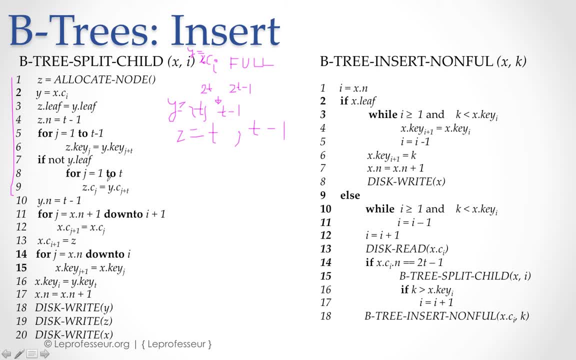 Basically, these are creating a new node z and giving it the largest t minus 1 keys and corresponding childrens of y. Very simple, line number 1 to 9.. And then line number 10 is adjusting the key count, key count for the original children. 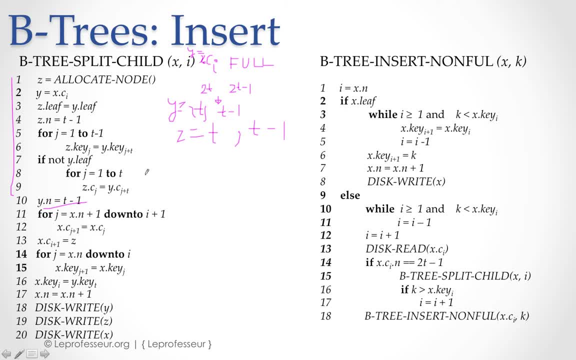 because now we have split it into 2 nodes, So we do not have. We do not have those many childrens now in the original one, Now 11 to 17,. these 11 to 17, line 11 to 17, these are inserting this newly created children z. 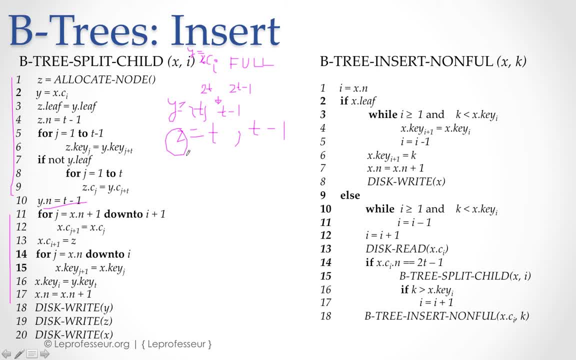 into the x, which was the parent of the y, And also moving the median key to the keys of the x in order to separate y from z, And adjusting the x keys count. And now line number 18 to 20, basically, these are writing the disk pages. 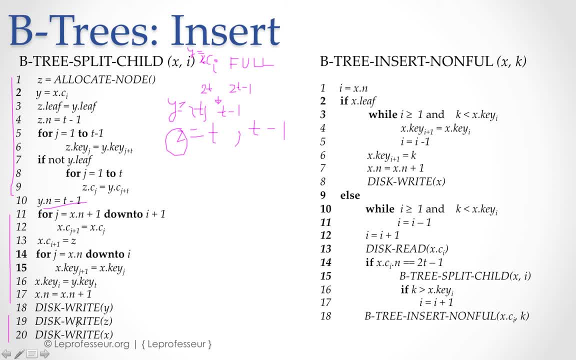 These operations are writing to the disks the information which is changed for y, x and z. Okay, So essentially, remember we discussed about that. b-trees are mainly used for secondary storage devices. That is why these operations are coming here. 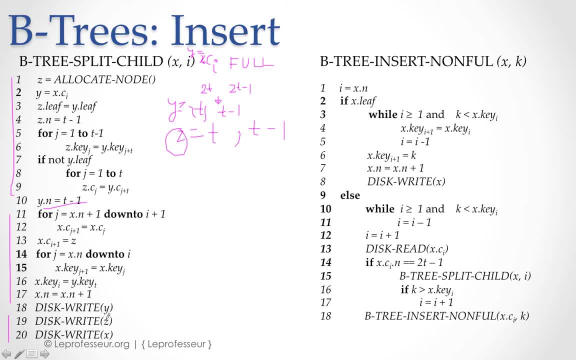 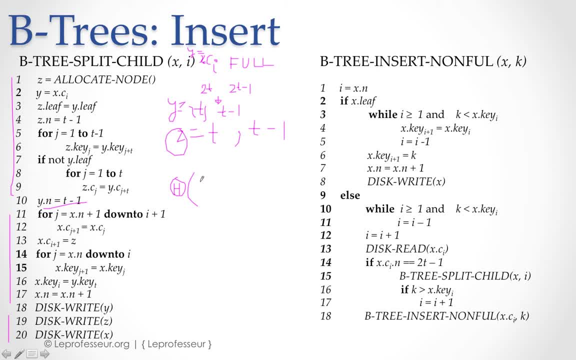 I am sorry. Remember we discussed about big O notations when we discussed about time complexity of an algorithm. So in this case it is going to take theta h time And all these disk operations are going to take order of one time. 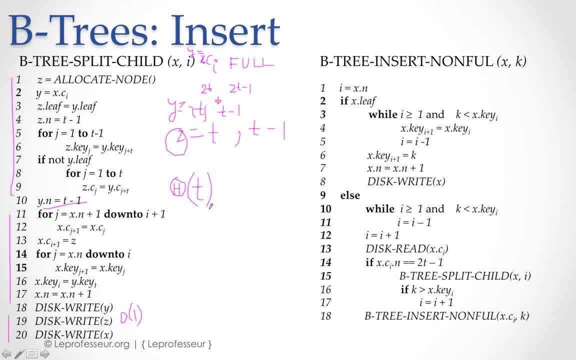 Where t, t is nothing but the order of meaning. order of b-trees. Okay, Now let us talk about the order of b-trees. talk about insert no full, okay, so when they, when, when our node, where we want to insert. 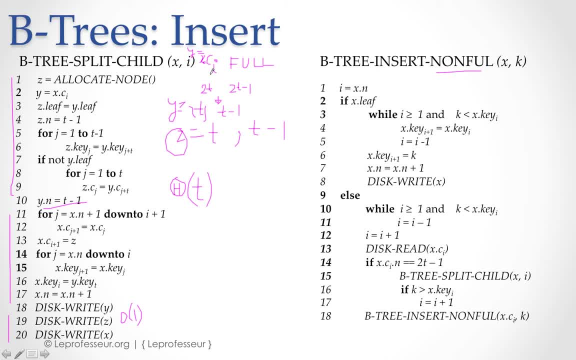 a key is full, then we have to split after splitting. okay, after splitting we have a node which is not full, so we use this procedure. no full at a node x and we want to insert key k, okay. so line number three is simple, that we're going to check whether x, that node, is leaf node. 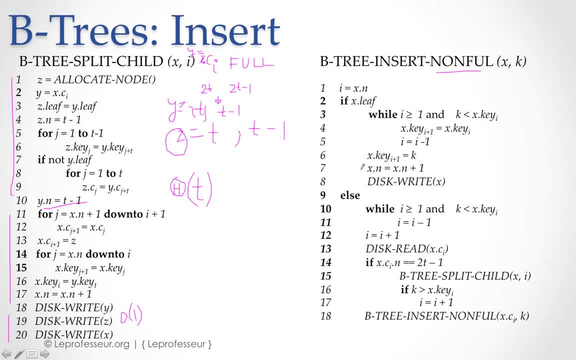 or not. if it is a leaf node, then we execute this procedure. if it is not leaf node, then we execute slightly different process. okay, so if it is a leaf node, we just directly insert. we don't have to do anything much. we we insert the, the key at the appropriate position. 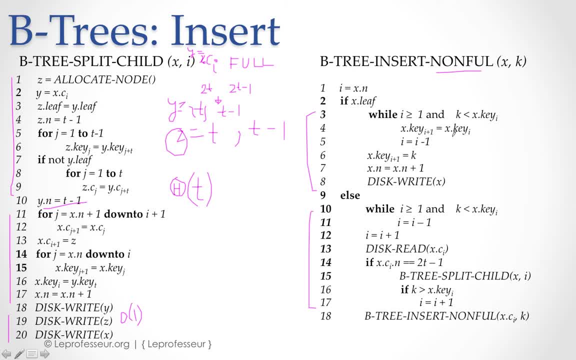 okay, but if, if it is not a leaf node, if it is internal node, then then what we do? what we do, we determine first which is the children of that intermediate node we want to insert. okay, and we read that children's information. okay. now same thing after we read that information. 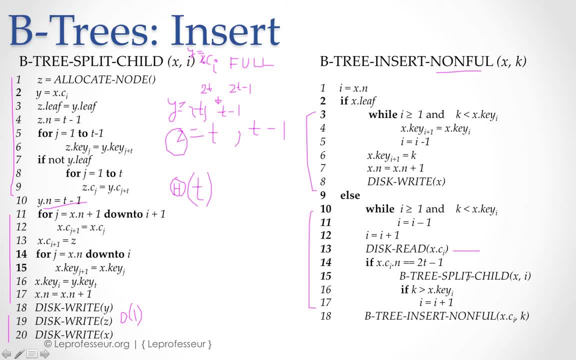 about that. children. we need to know whether this children is full or not. if it is full, then we actually split the children and after splitting we use the same routine recursively. right, isn't it simple, fascinating technique- how to use recursions. okay, now think about how much time. 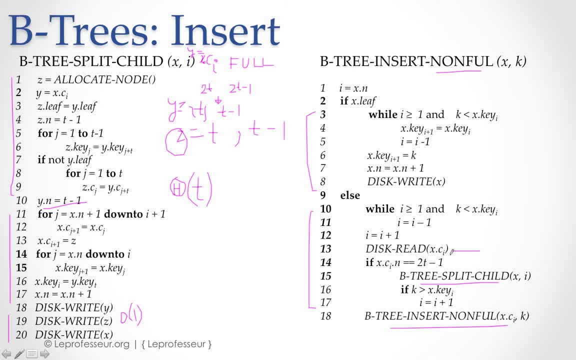 and this will take, now, this, this disk, access to read the page. how much time is going to take? it's going to take, whatever is the height of the tree, and how much this, this total whole process, is going to take, to insert key at a node which is not full. again, it's again simple order of T, which is 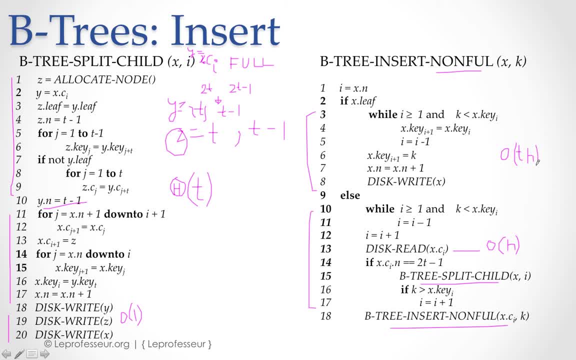 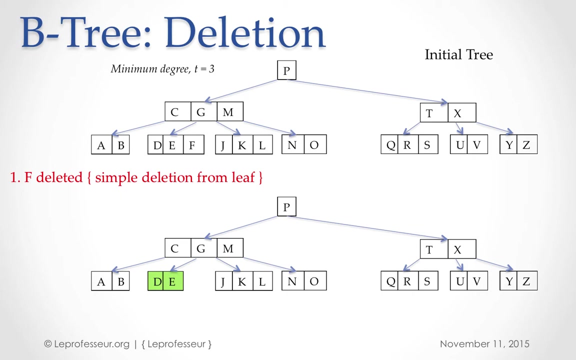 the minimum order of the tree and the height, H. okay, we can also write it as T. H is nothing but log base T and N. all right, okay, so we discussed about insertion processes. Now deletion is how to delete the key from a b tree. this is a bit complicated and a tricky procedure, so we're going to. 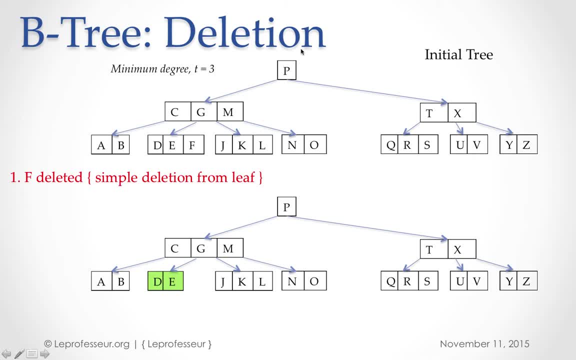 discuss in different cases. let's say we have been given a, a tree, B, three. okay, this is the originally given bitwee. alright, now case number one: we want to delete a, a key, f- okay- from a node, and this node is a leaf node, okay, so we just simply delete f. 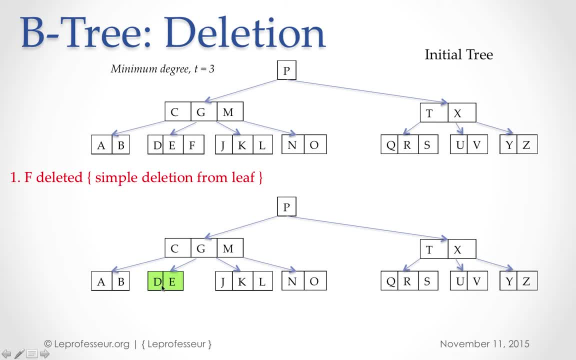 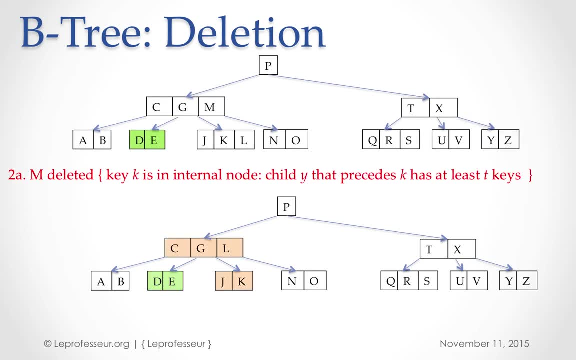 and you know, after deleting f, we just left d, e, the keys at this node. very simple. now let's talk about another case in which a key- k- is in the internal node. so we want to delete m. okay, you want to delete m which is at internal node and the child which precedes k, okay. 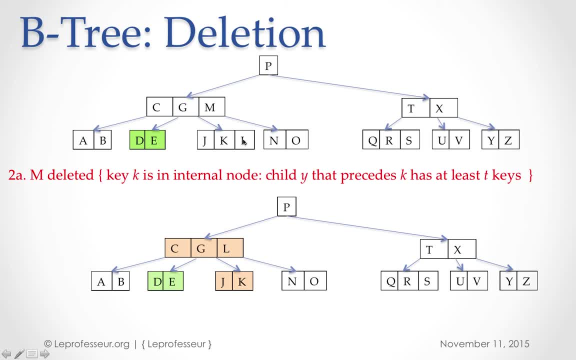 the child which precedes k has at least key t keys. now we already said that we have this tree. uh, on, minimum order is three, so it has three keys. so what, what we're gonna do in this case? so we want to delete m. we have deleted m now. 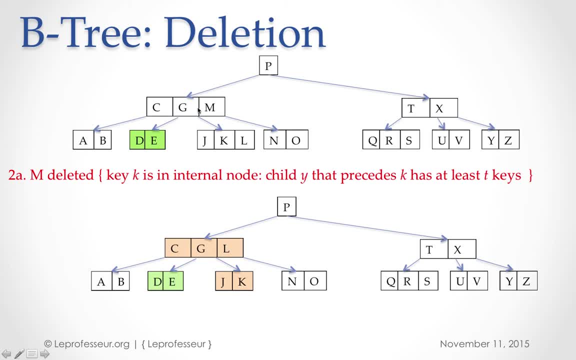 after deleting m, uh, we, we are left with two keys here, and so this, this is basically, uh, so moving, um disturbing the b tree property, so what we're gonna do? the child which is preceding this m? okay, the right, uh, most key, or the greatest key, l? 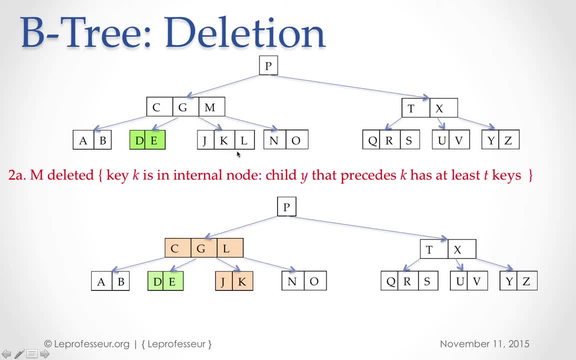 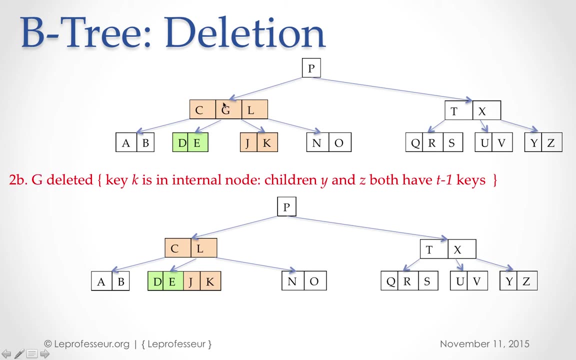 will take the place of the m. so we move m, l in place of m, and the resultant tree would look like this: okay, now let's take another case. so in this case, what we did, uh, was we want to delete g. okay, so g. this is a case where k the key is, which we want to delete. 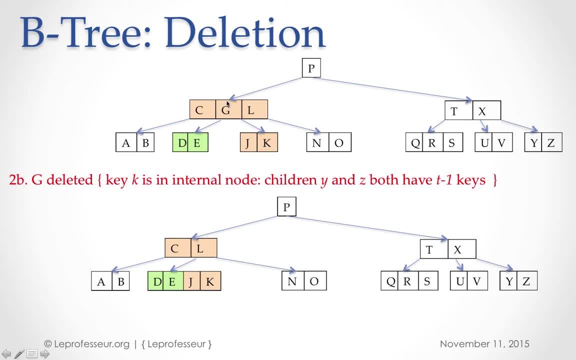 is present in an internal node, okay, and the children y and z- both children will have t minus one keys, okay. so what we're gonna do in that case to preserve, uh, the bt property? uh, also, after deleting the key, what are we gonna do? we merge these two children, y and chat. we merged and we removed this key. okay. 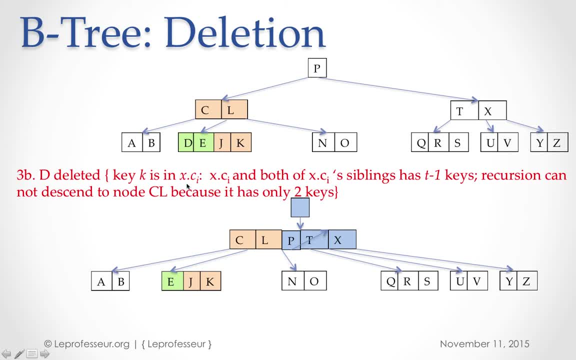 now let's talk about another case. okay, so don't go with the with the 3b or 3a. i'm discussing 3b first because i'm maintaining the consistency with the textbook. okay, now 3b, we want to delete d. okay, so d what what? it means that the, the key, is not at this internal loop, but 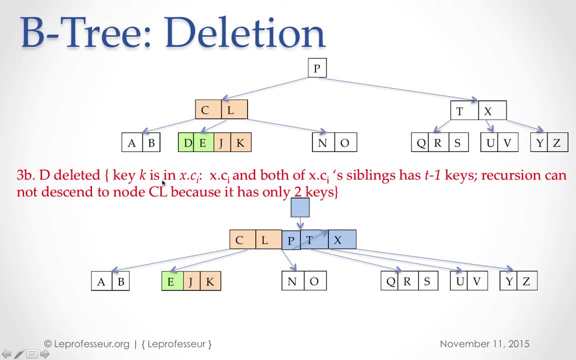 at the children, at the children node x dot c i at the particular index i. okay, now. now x dot c i and both of x dot c i siblings have t minus 1 keys. okay, so now what happens in this case? the recursion cannot go beyond this point, because this c 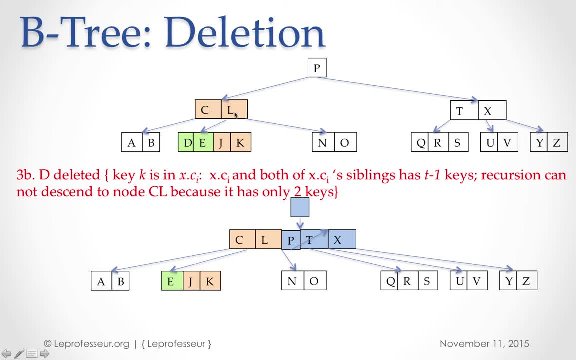 in l. it has only two keys, so to go recursion beyond that, we need more than two. so what we're gonna do, we're gonna merge. we're going to bring the key which is of its, its parent, with this and merge cl with the tx. okay, so we merged cl, dx and we wanted to delete d. now we can delete d. t is gone, okay. 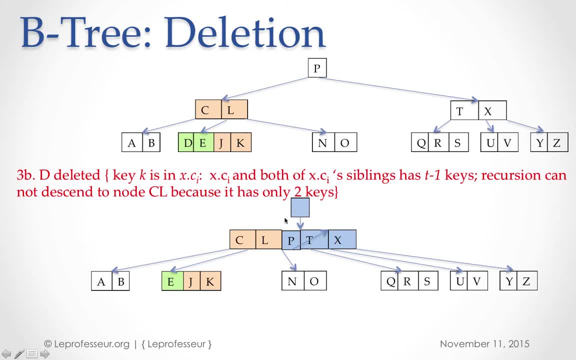 and result entry is like that: now our root is empty. the root is empty. we just need to write root empty. there is no key in the empty, so we can simply make a new root of the tree, which is CLPTX. this node becomes the new root of the tree and the tree height is: 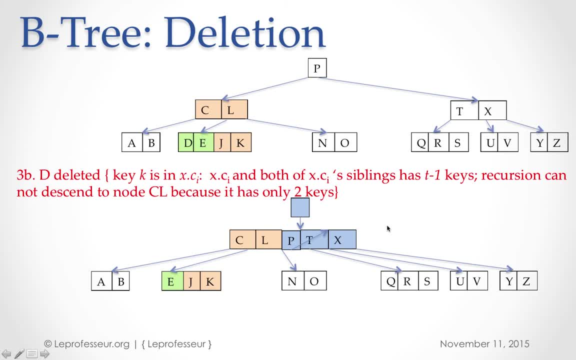 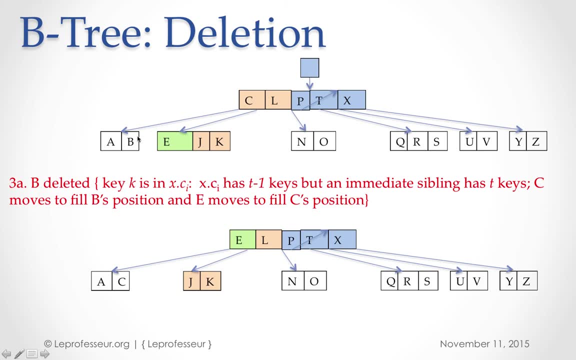 decreased by one. ok, now let's talk about another case, 3a. ok, now it is a similar case. we want to delete b. ok, very similar case to the previous one, with a little difference: that that the children has t minus 1 keys. ok, star ci has t minus 1 keys, but immediate sibling. so in the previous one. 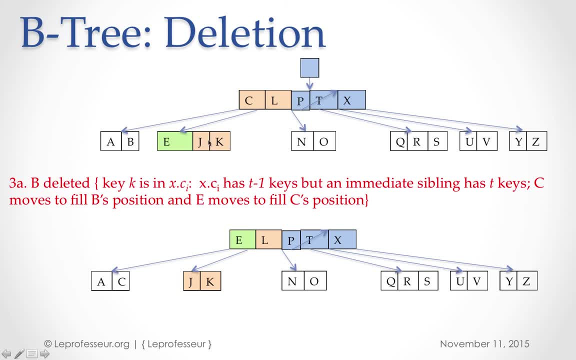 immediate sibling is this one has t keys, means 3 keys. ok, so now what happens? that when we want to delete b, ok, so the C, which basically comes after this key, because it's the leftmost children in this case, what happens? the C takes the place of b, b is gone. and now this: 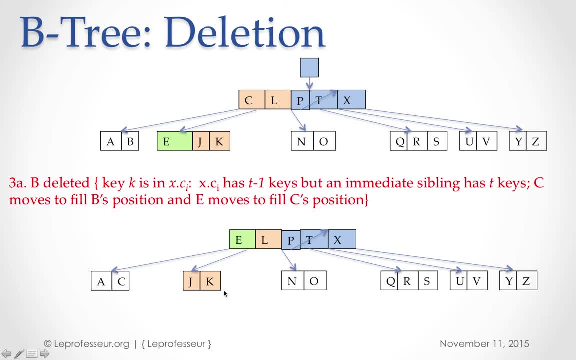 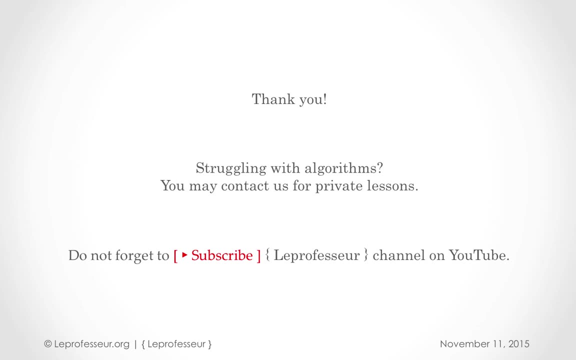 e takes the place of the C, ok, and resultant tree will look like this: ok. so, guys, this was this was a. this was a quick video on basic operations of on on b trees. if you want to implement these algorithms, I would recommend you to do so. you can take any programming language- ideal would be the C or C++- and get your. 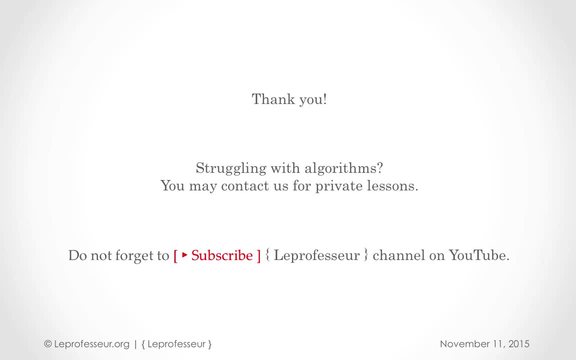 hands dirty. thank you very much for watching this video. if you are struggling with algorithms, you may contact us for private lessons also, we are. we would be happy if if you subscribe to our channel. Thank you very much. Lee Professor's channel on YouTube. This encourages us to to create more. 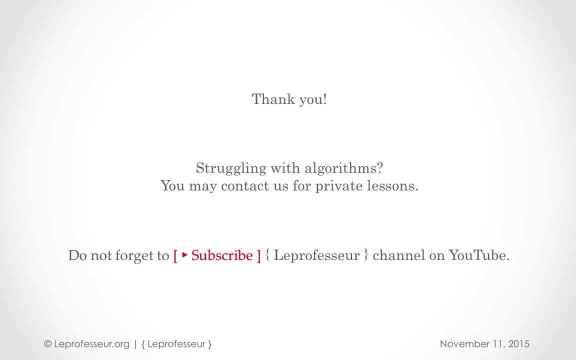 interesting videos and also do not forget to to write your comments, which makes us to realize that, okay, we did this mistake. with that mistake, and help us to improve videos going forward. Have a wonderful day. Thank you once again.